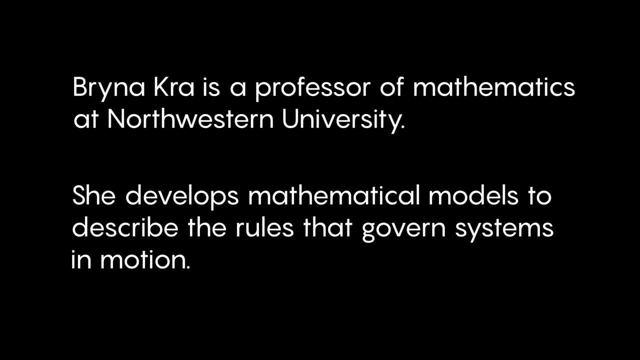 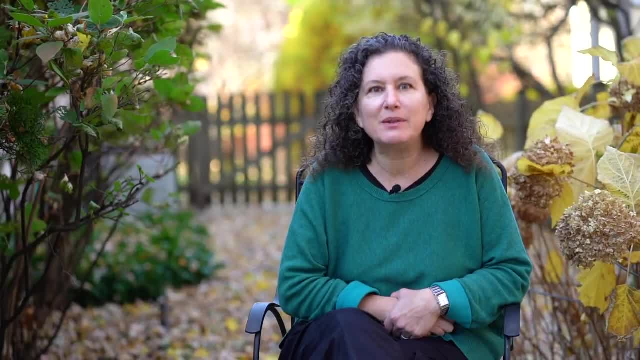 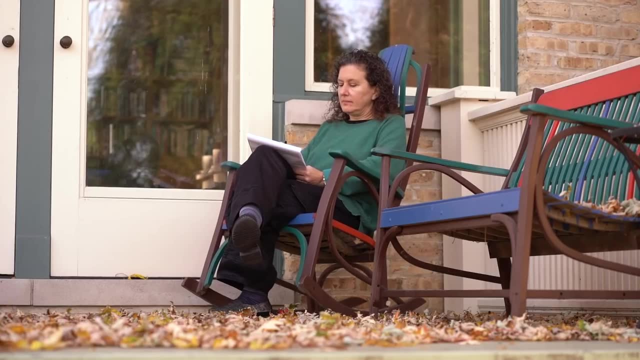 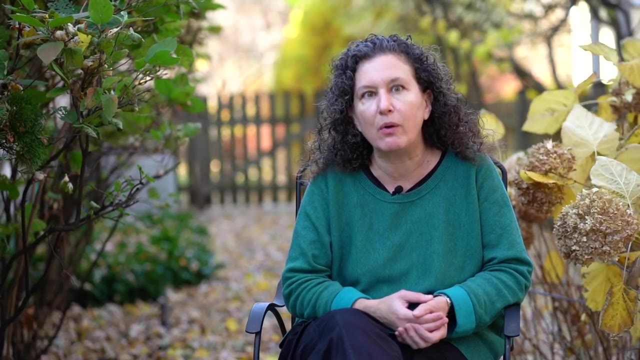 I work in dynamical systems. What a dynamical system is is a space with a bunch of rules on it that tell you what happens to each point in that space. What I want to do is then be able to predict long-term behavior about what happens to this system, as you keep applying that rule over and over. 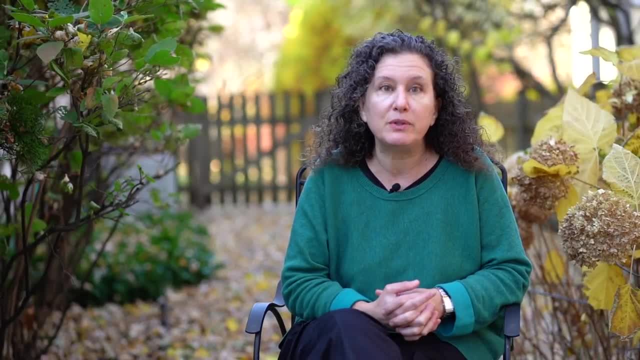 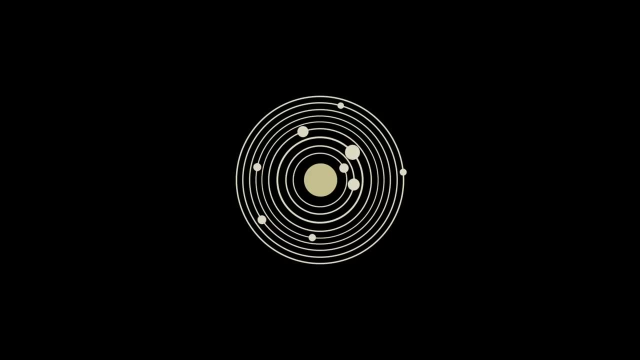 This kind of space. the ones I look at are very abstract, but you could think of them as something like planets rotating around the sun. You take a snapshot where each one is once a second and then try to tell me where they will be millions of years into the future. 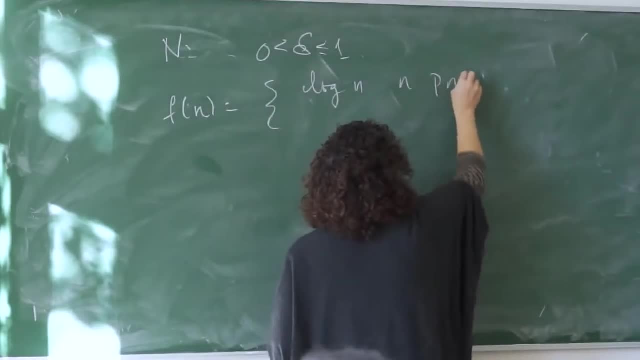 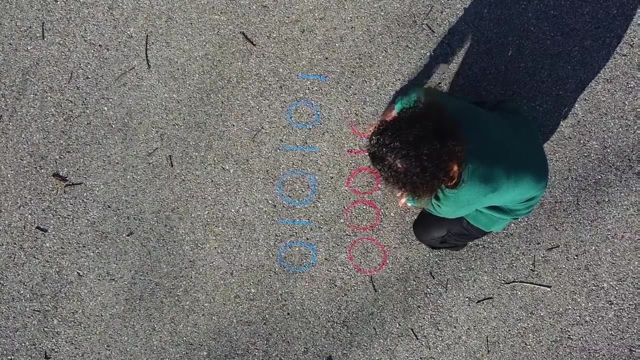 One of the tools I use in my research is symbolic dynamics, and what this is is a mechanism to take a complicated, abstract dynamical system and recode it in a simpler way so that we can study it. Let's say, you're standing and observing a traffic light. 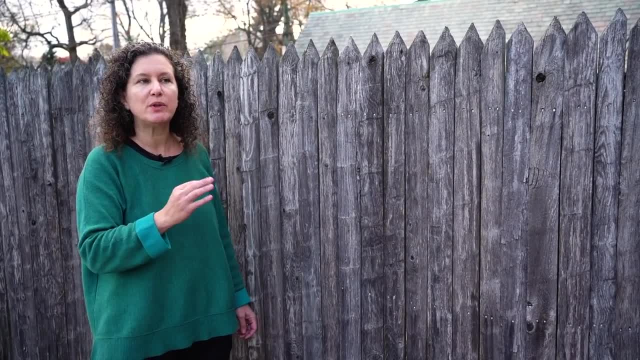 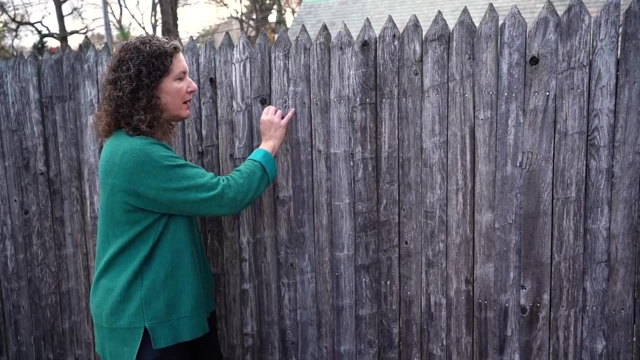 And I'm going to pretend there's no yellow. to make it simpler, It just alternates between red and green, And let's say it changes every 30 seconds. And every 30 seconds I might write down the color of the traffic light using a 0 to say that it's red and a 1 to say that it's green. 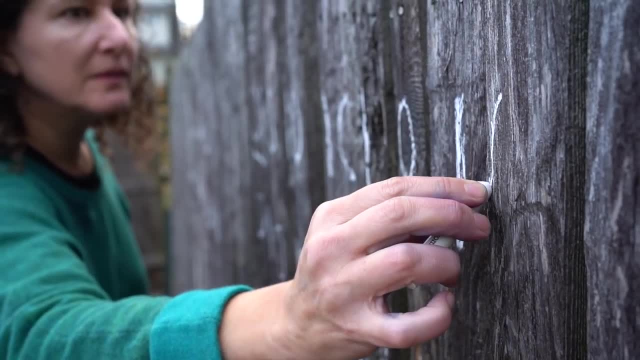 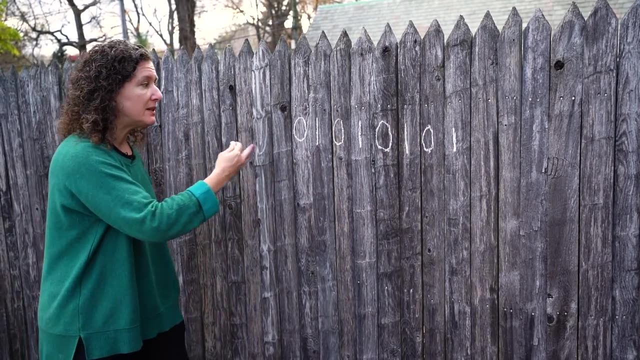 And my pattern will just say 0, 1,, 0,, 1,, 0, 1, and it will continue like that forever more. In other words, this is a super simple pattern, because it's just this little block of 0 and 1.. 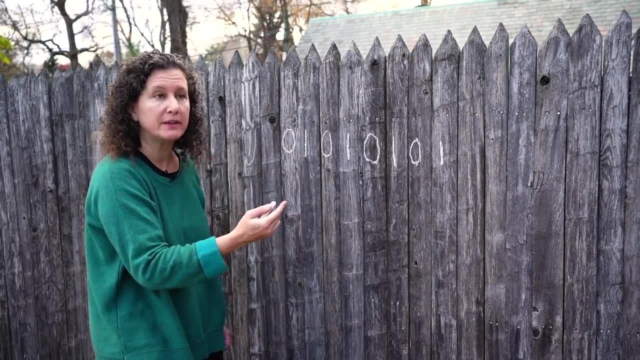 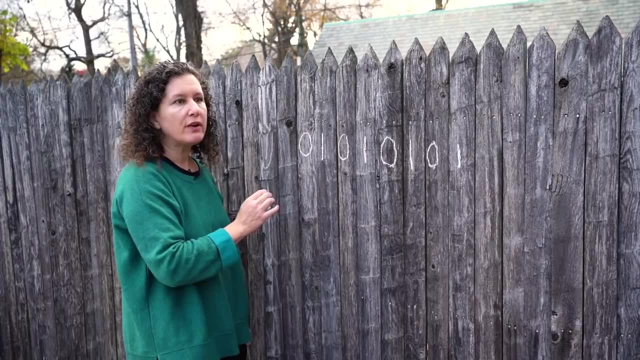 Repeat it all the time. It's a periodic pattern. Now, let's say I look at that same traffic light, but I don't measure it every 30 seconds. Maybe I measure it every 31 seconds or every 32 seconds, And when I do this I might see the same number in a row twice. 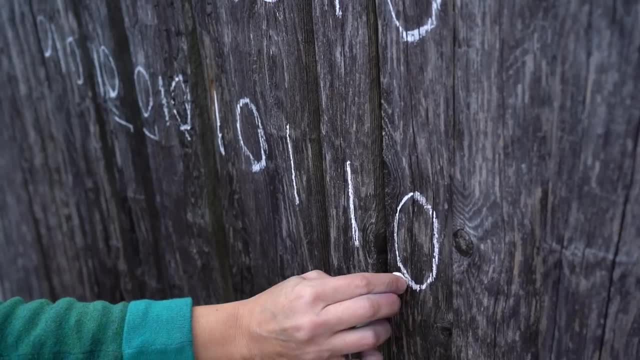 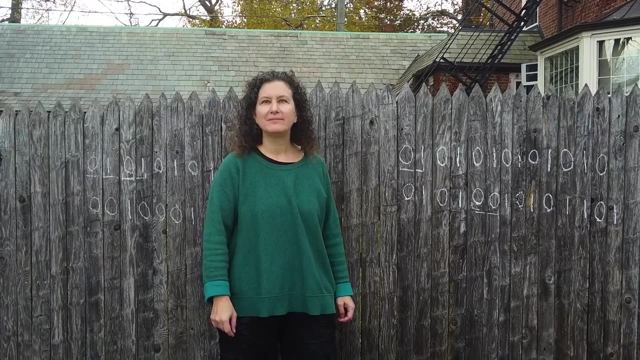 So this is something that I can detect using symbolic dynamics. It's really a beautiful part of math to find connections which are not apparent And finding structures where you didn't know that they existed, Where you didn't know that they were going to be there. 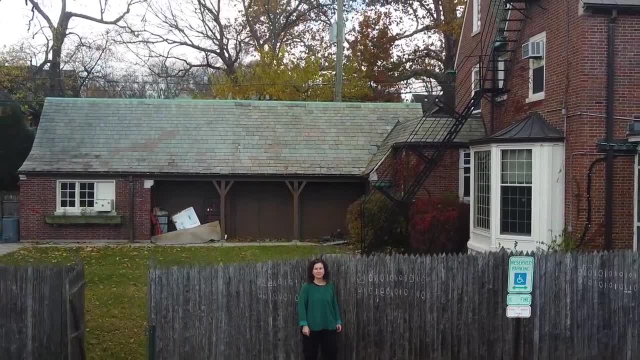 To me, this is one of the best parts about doing research.